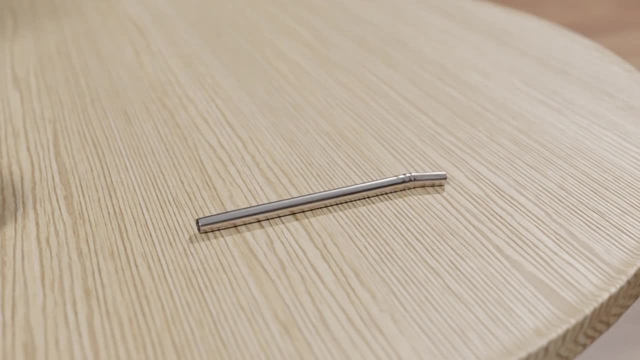 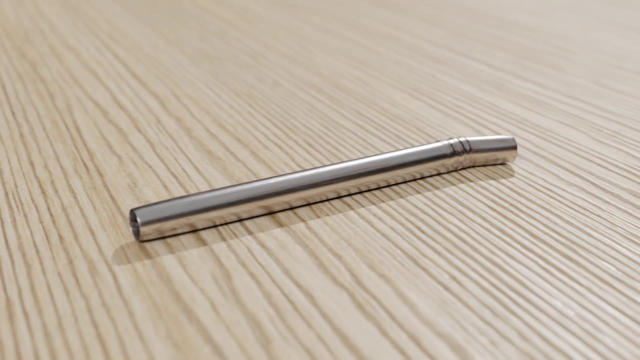 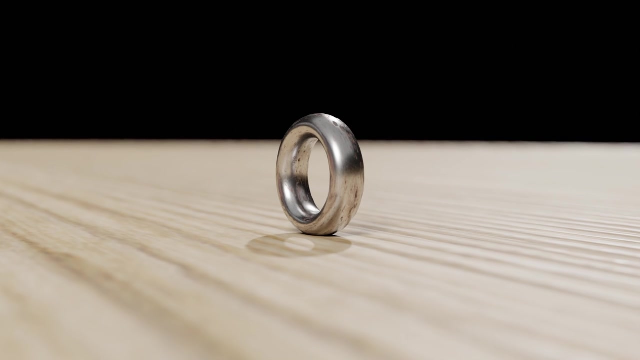 straw have. You might say it has two holes: one where the liquid comes out and one where the liquid is sucked in. But imagine if we made a straw shorter, and by short I mean really short. At this point the straw looks just like a doughnut and it clearly has one. 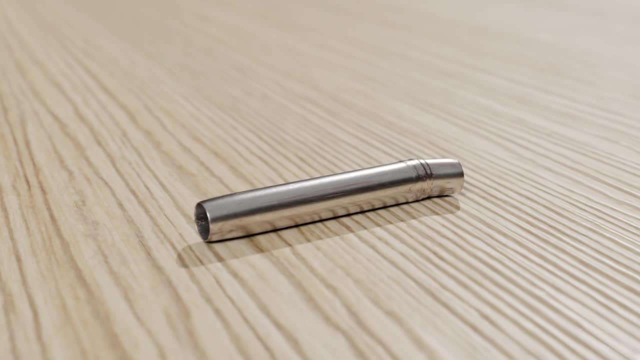 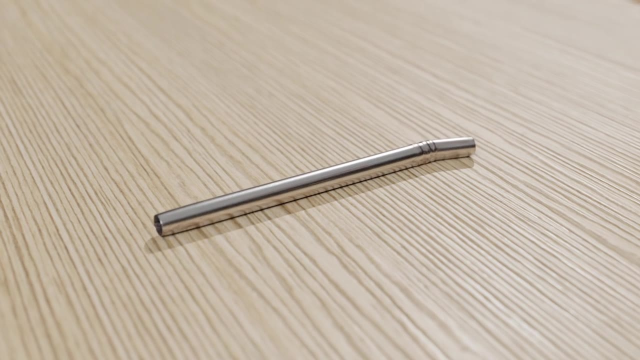 hole When we reverse the process. is there ever a point in time where it stops having one hole and suddenly has two holes? If it did, at what point during this process did we ever cover up a hole, reducing the total number of holes from two to one, when all 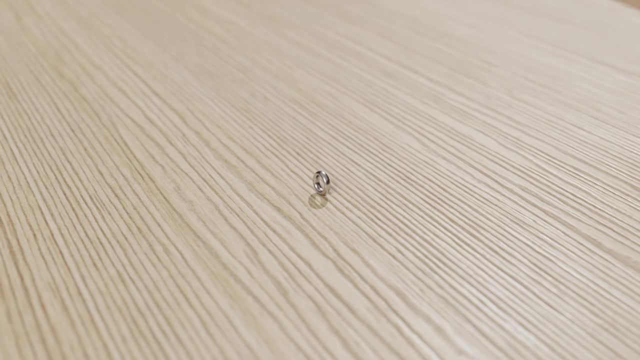 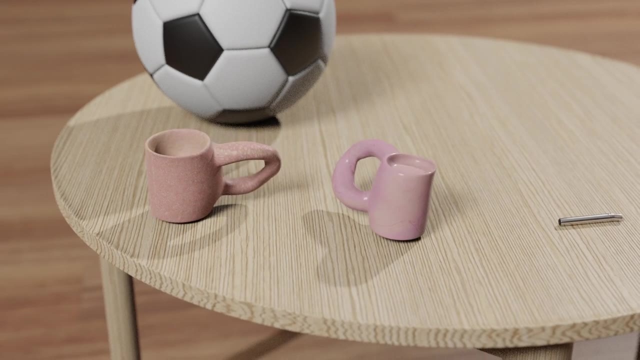 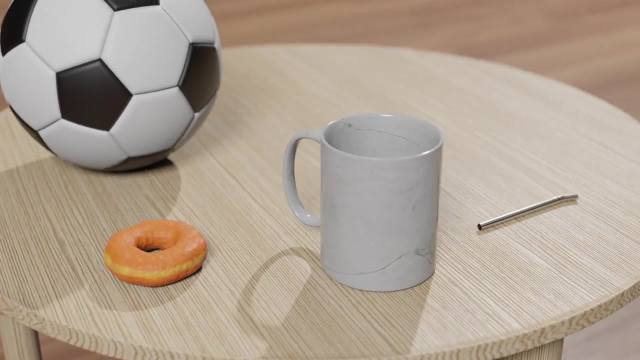 we're doing is continuing, In fact, to a topologist. a doughnut, coffee, mug and straw are the same. They all have one hole and are said to be homeomorphic to each other because we can continuously deform one into the other. However, a doughnut would not be homeomorphic to a ball If we try to. 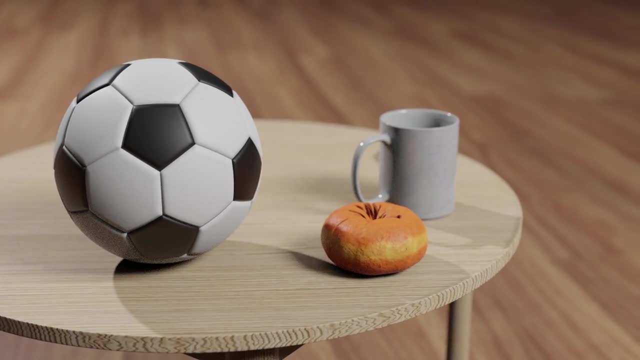 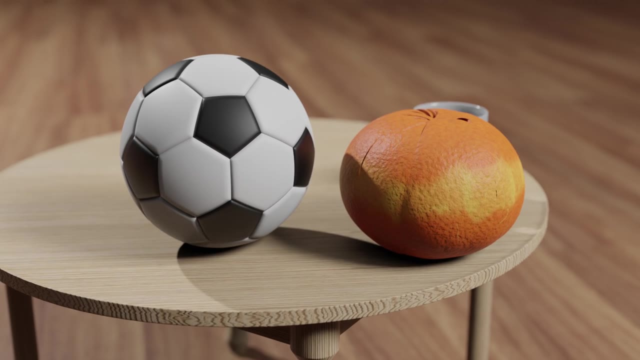 continuously mold a doughnut into a ball by pinching the hole away. there will always be a point in time where it suddenly stops having a hole. so it is not a continuous deformation and thus a ball and a doughnut are considered not topologically the same. 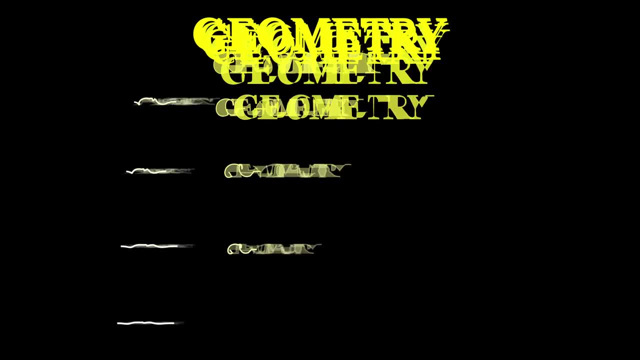 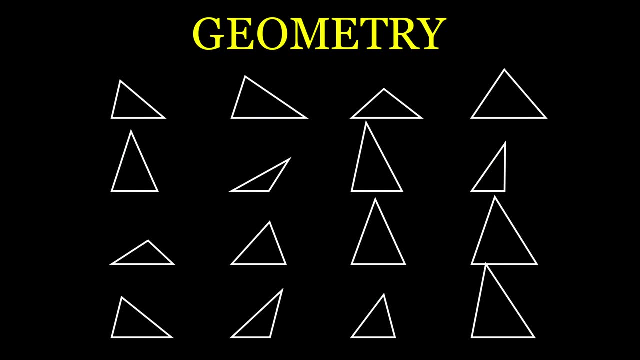 In the familiar realm of geometry, on the other hand, lengths, angles and scales all matter, so these triangles would all be different from its point of view. In topology, however, not only are all triangles the same, they are the same as any circle or square, precisely. 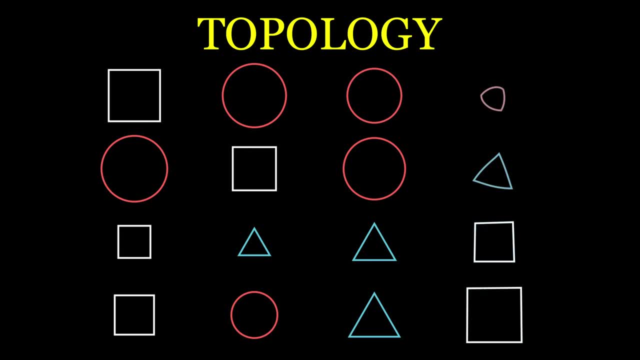 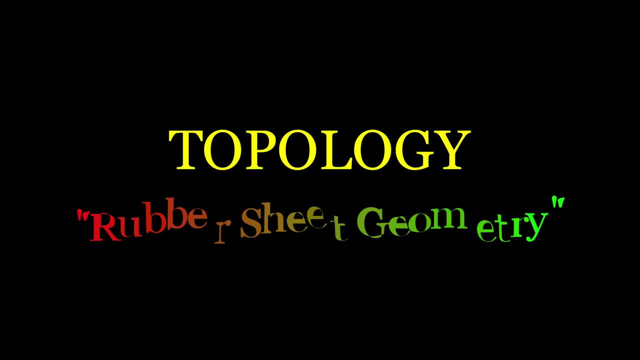 because we can continuously deform them into each other without causing any problem. So let's get started cutting or gluing, as if shapes are made of infinitely flexible and compressible rubber. This is why topology is also known as rubber-sheet geometry. 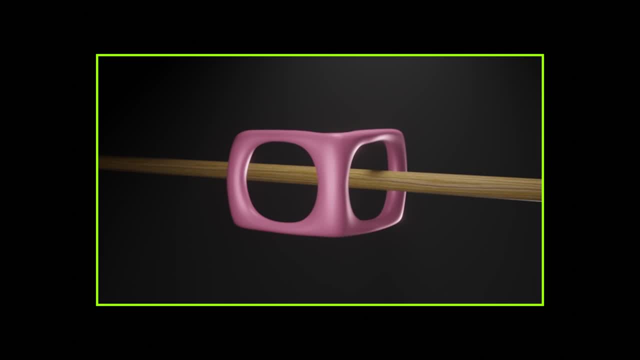 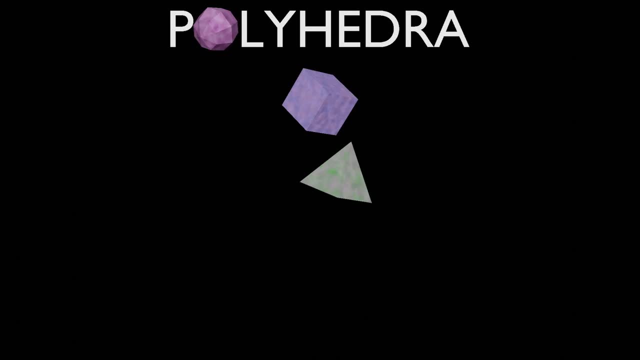 In a moment we will explore a fun, counterintuitive puzzle in topology, but first we'll look at a type of 3D shape known as polyhedra. What do a cube pyramid, dodecahedron or any other 3D shape with flat faces have in? 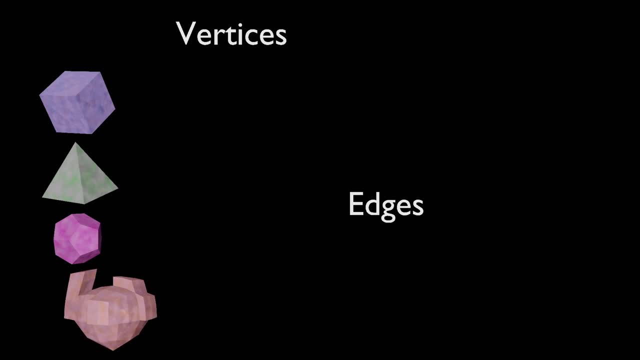 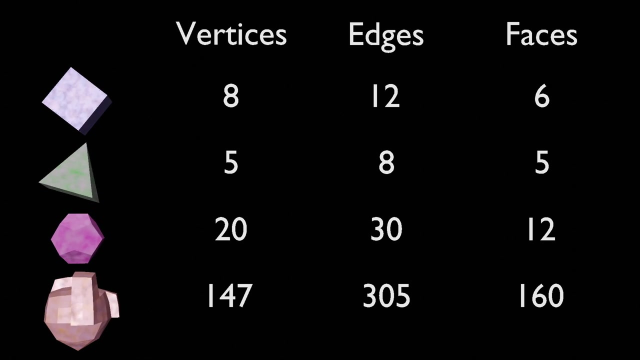 common. Well, consider how many vertices, edges and faces each polyhedron has. The cube has eight vertices, 12 edges and six faces. Counting the values for the rest, this is what we get. Can you find a pattern? 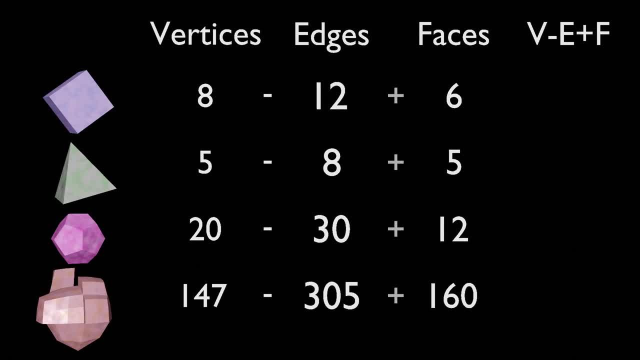 As it turns out, the number of vertices minus the number of edges, plus the number of faces for each shape is 2.. This called the Euler characteristic of polyhedra. specifically, 2 is the Euler other characteristic of any simple polyhedron, which is just a solid figure with flat faces. 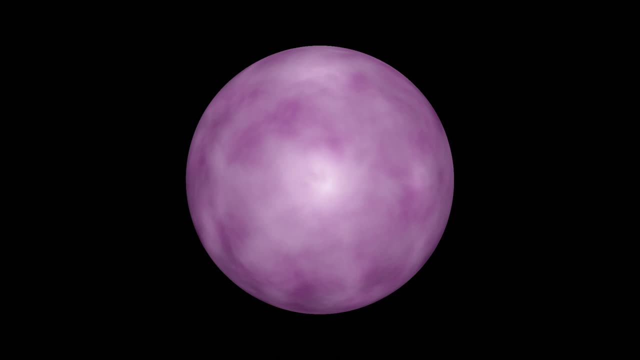 But what about a sphere? It doesn't have any flat faces. so what could this other characteristic be? To answer that, consider this 3D shape. This is just a simple polyhedron, so it will have an other characteristic of 2.. When we add subdivisions to the shape, it will still have an other. 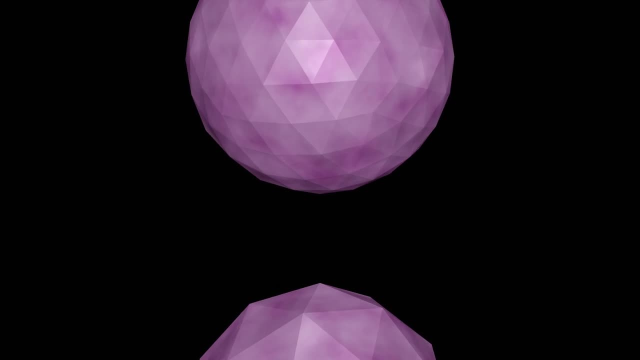 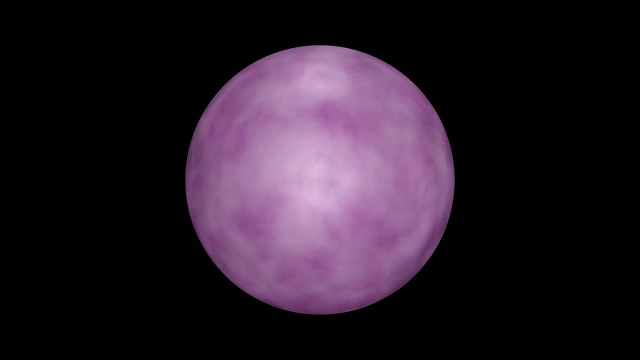 characteristic of 2.. But as we add even more, the shape will gradually approach that of a sphere And at an infinite number of subdivisions this thing will literally turn into a sphere. But we know that regardless of further subdivision, the Euler characteristic remains 2.. 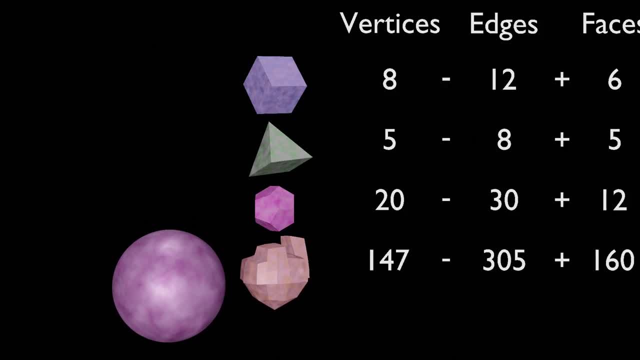 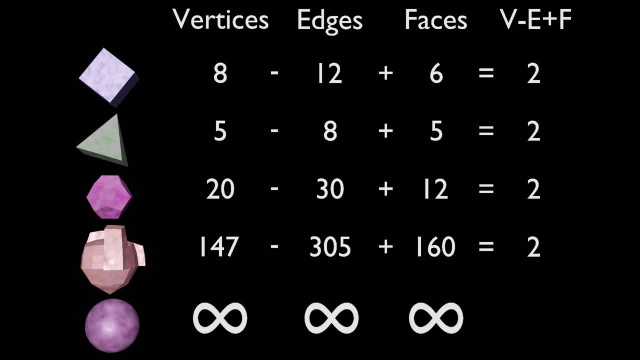 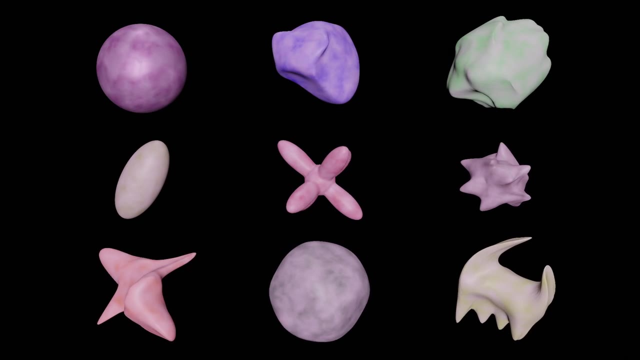 It appears that the sphere is just like any other polyhedron, but with an infinite number of vertices, edges and faces, And yet its Euler characteristic is still 2.. Isn't that cool? And this thought process applies to any 3D shape with smooth surfaces that are based on simple 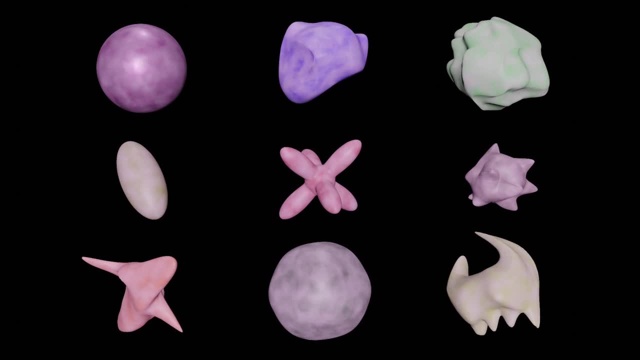 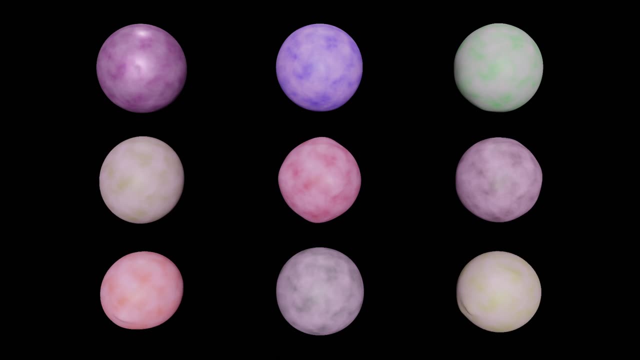 polyhedra. As a result, every one of these shapes has an Euler characteristic of 2.. And, as it turns out, we can continuously deform any of them into a sphere. In other words, if two objects are homeomorphic, then they have the same Euler characteristic. 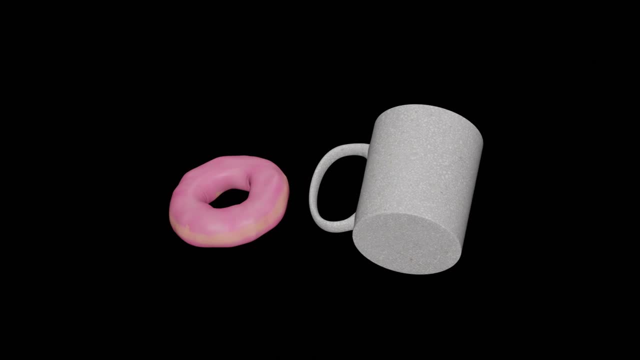 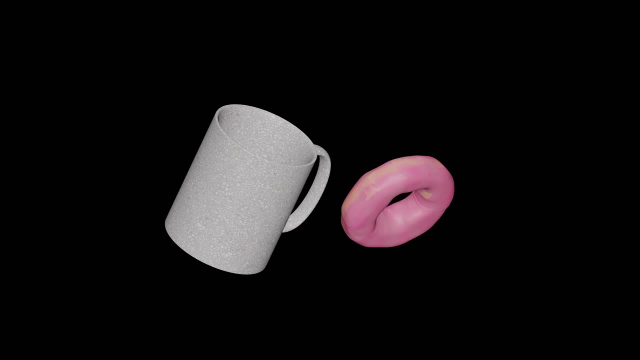 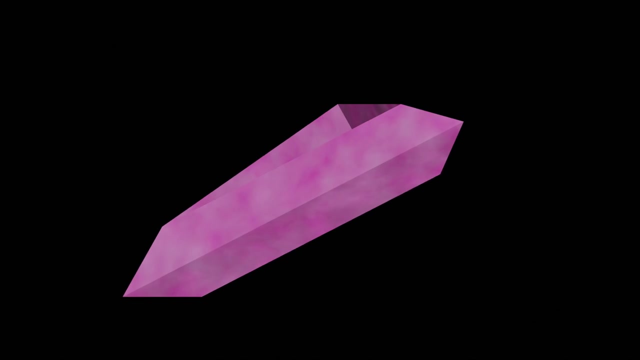 But what about torus-shaped objects such as a mug or a doughnut? We can compute the Euler characteristic of a torus in the same way we did before, by finding a simpler version with flat faces. Take this shape, for instance. It has one hole, just like a doughnut or a mug, but we can now easily compute its Euler characteristic. 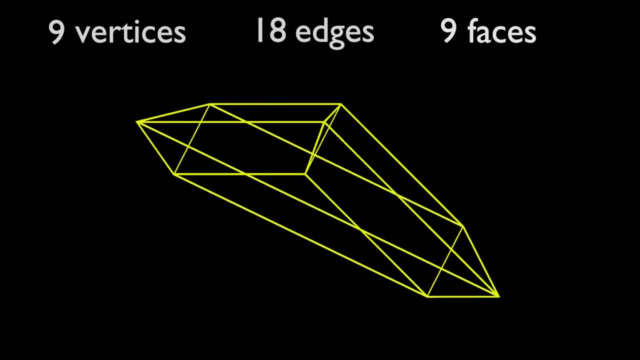 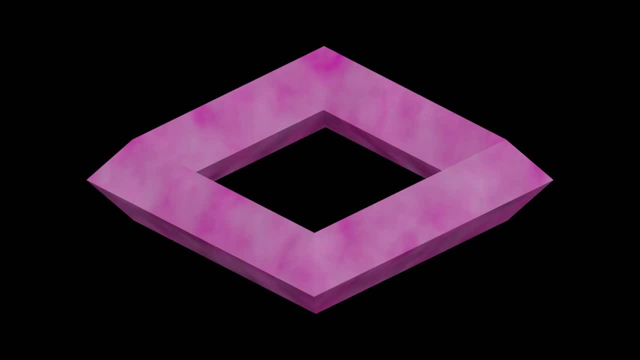 It has 9 vertices, 18 edges and 9 faces. That gives us an Euler characteristic of 0.. When we add more subdivisions, the Euler characteristic is still the same. However, as we add even more, the shape will gradually approach that of a torus. 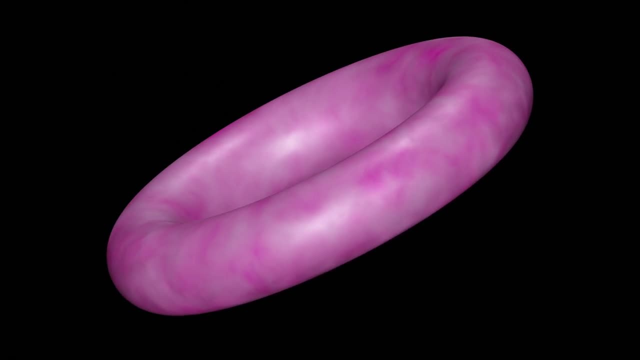 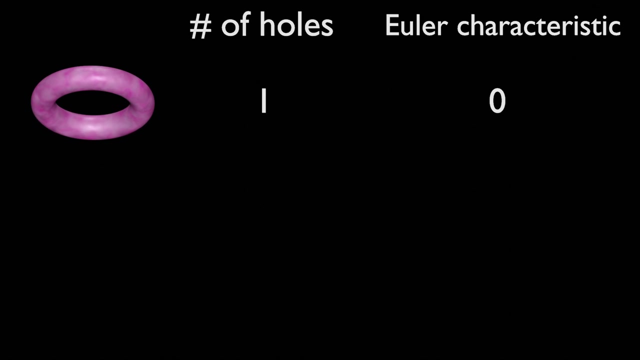 and with an infinite number of subdivisions it becomes a torus, And yet its Euler characteristic is still 0. At this point it appears that any object with one hole has an Euler characteristic of 0. For objects with two holes, the Euler characteristic is negative 2.. 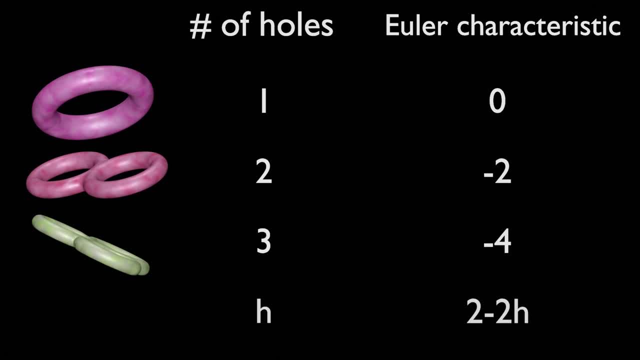 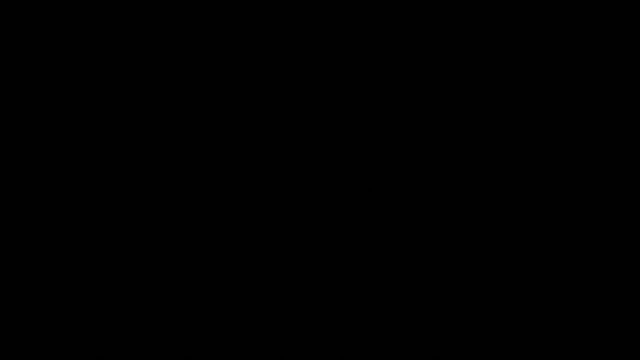 For three holes it is negative 4.. In general, an object with H holes will have an Euler characteristic of 2 minus 2H. Now the puzzle. Let's say there's a very long rod and we have this figure-8-shaped object. 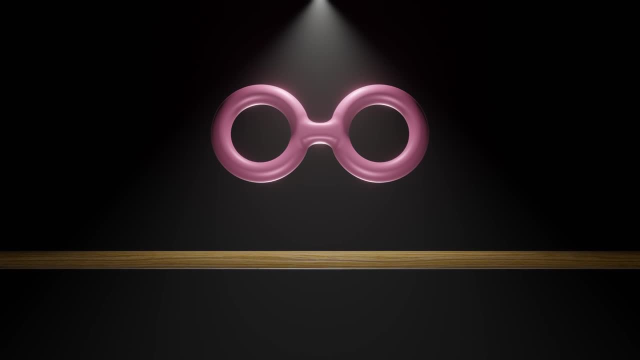 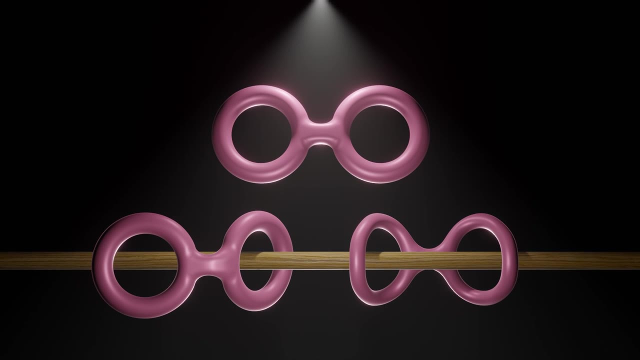 let's call it a handcuff with two holes. We can make the rod go through the handcuff in two ways. Either the rod goes through only one hole or it goes through both. Here's the challenge: Can you figure out how to continuously deform one handcuff into the other? 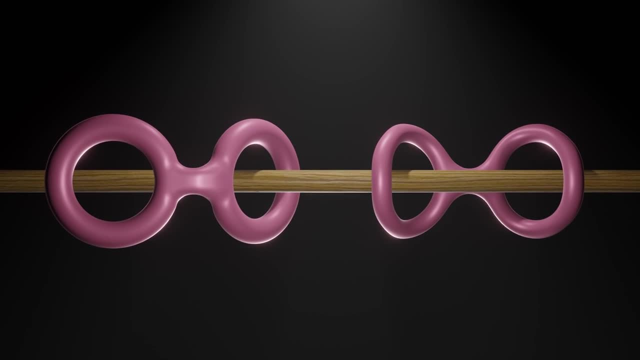 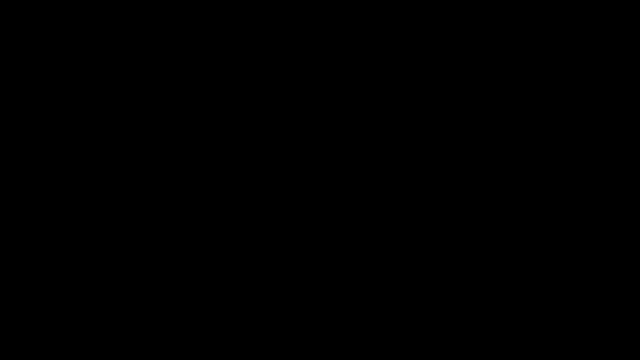 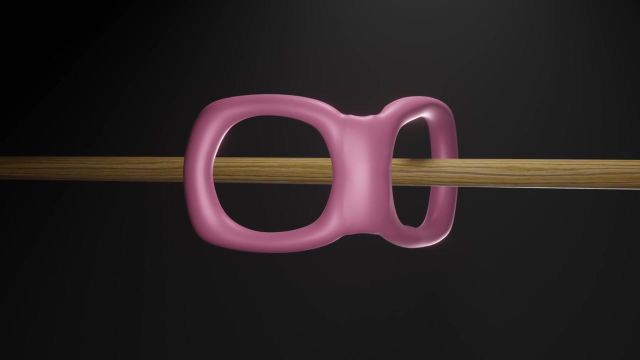 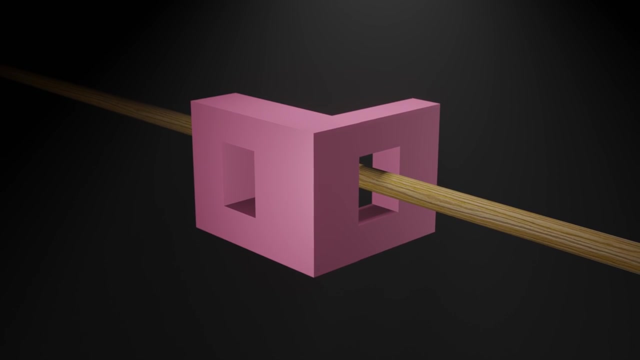 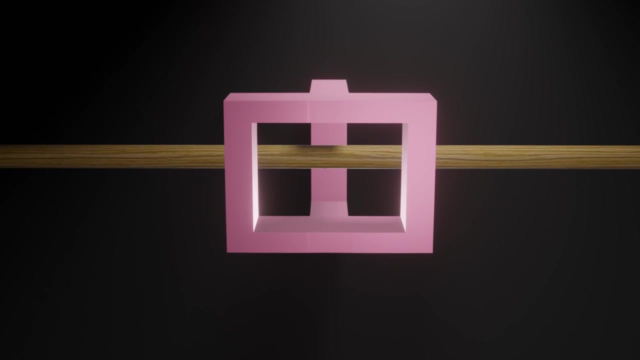 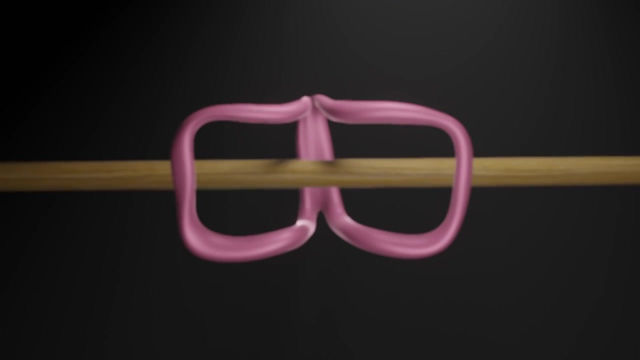 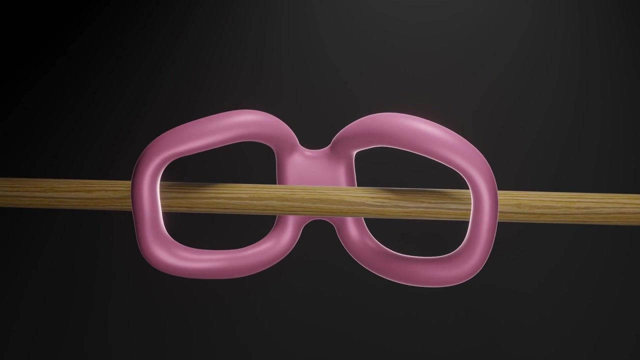 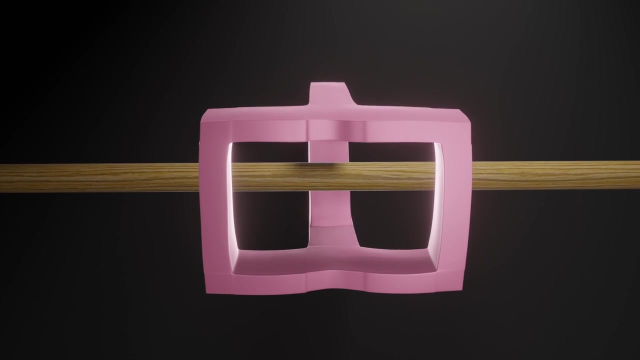 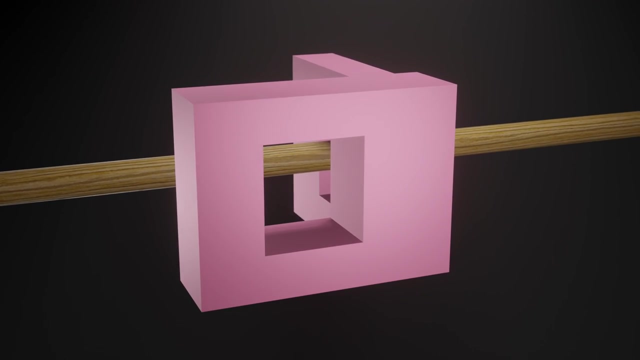 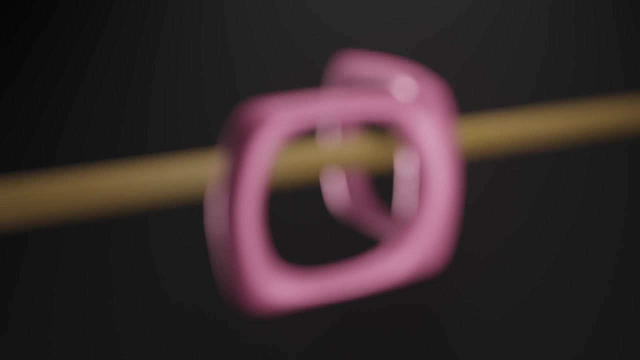 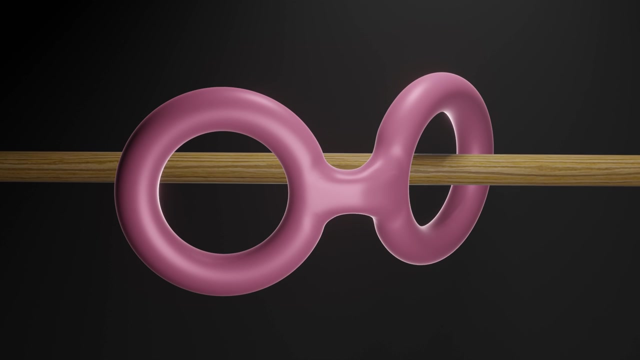 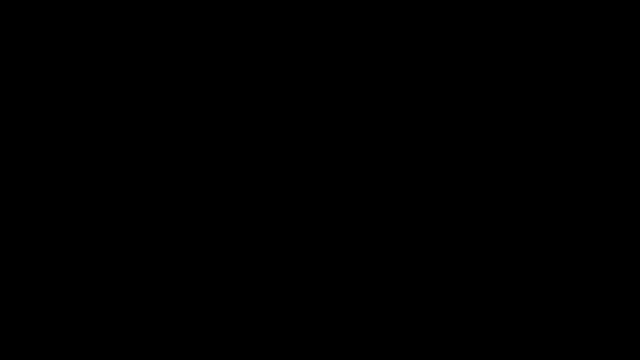 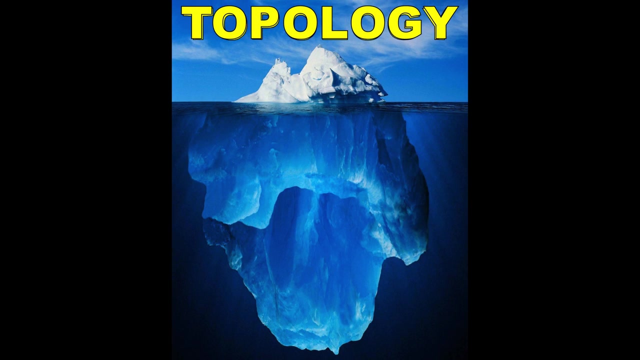 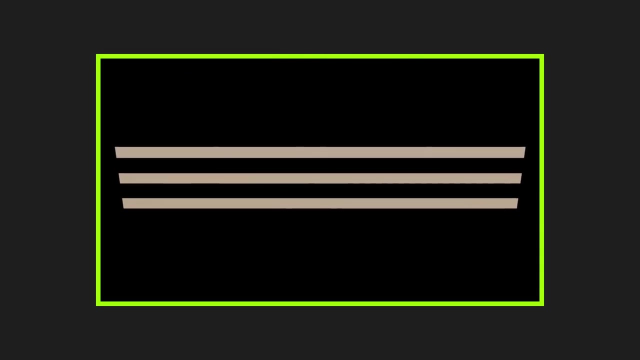 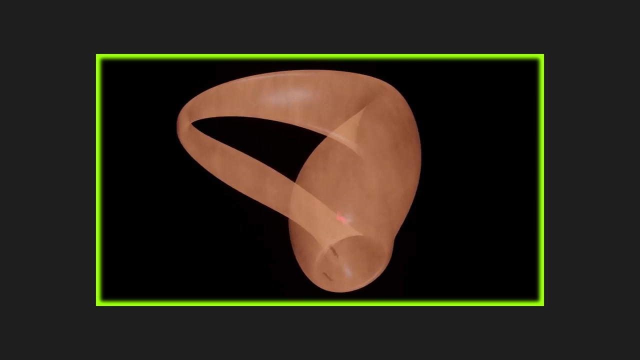 without removing it from the rod or doing illegal actions like cutting and gluing. Pause the video now if you want to think about it. F 23, 24, 25. Thank you, Thank you, And after that you can further satisfy your curiosity with Brilliant, which I'm happy. 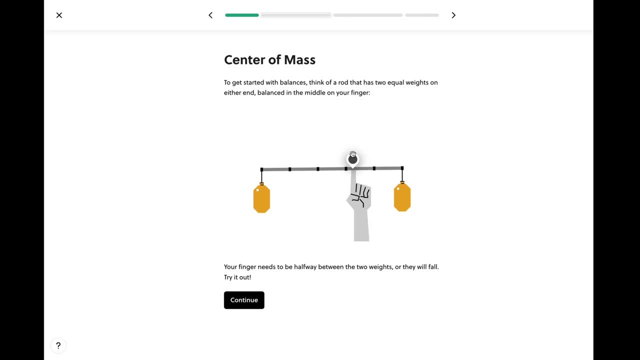 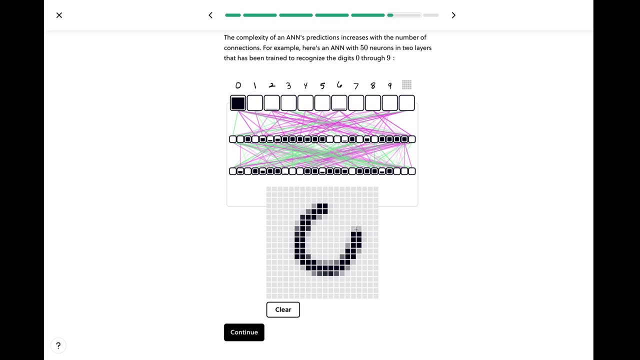 to say, is the sponsor of this video. Brilliant is a website and app that uses a hands-on approach to learning, with lots of interactive and engaging visuals to help you learn math, science and computer science. It makes use of active learning, which is perfectly tailored to the way the human brain